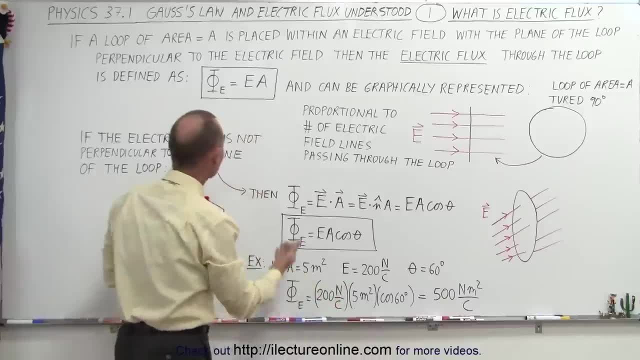 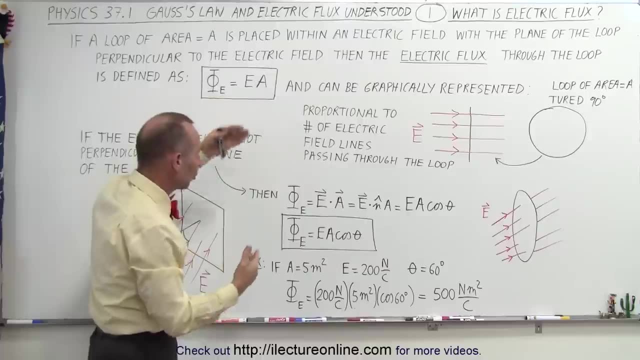 will go through the loop and you have more flux. so really the amount of flux depends upon the strength of the electric field and the size of the loop would be small or large. the amount of flux to the loop of course will depend to that. it'll be proportional to that area. so we can say: 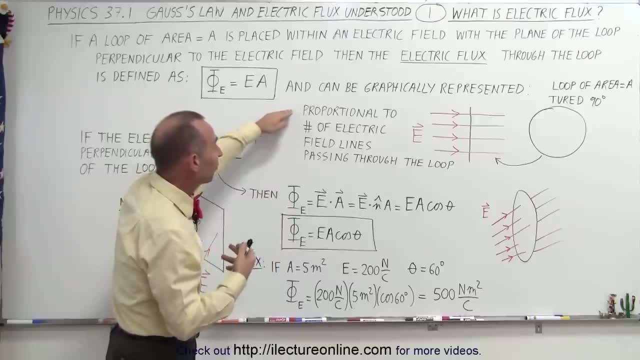 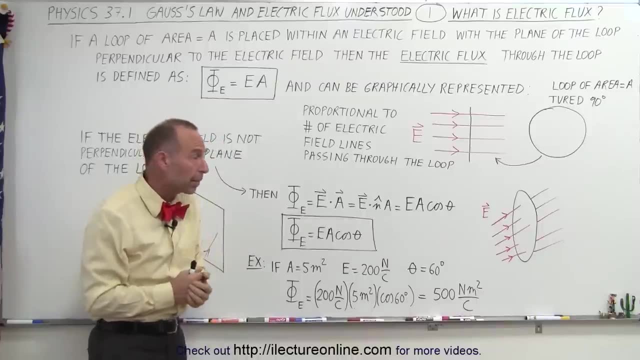 that we can graphically represent it such that the electric flux is proportional to the number of electric field lines passing through the loop, and that's probably the best way to think about it. what's also important is what happens if the electric field doesn't go to the loop. 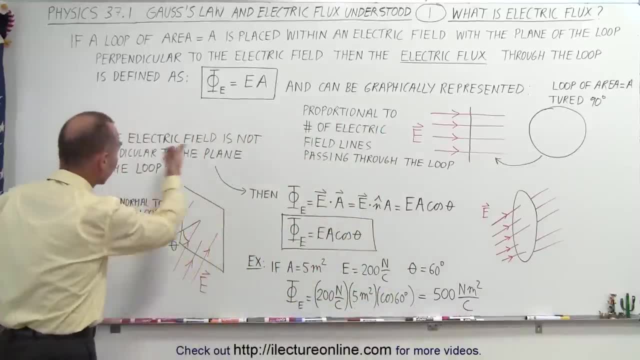 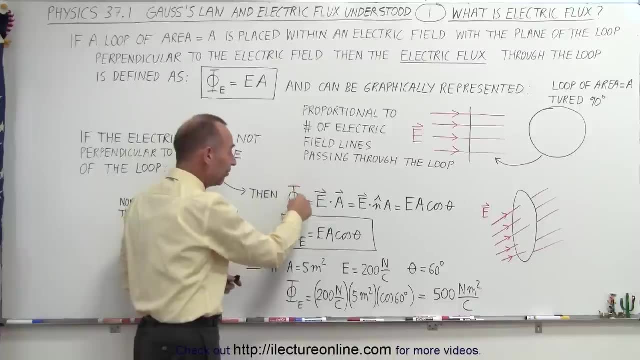 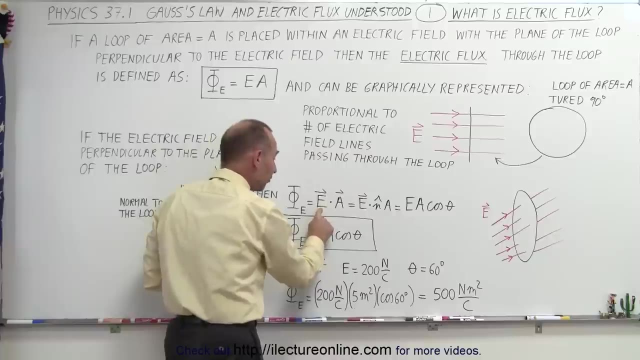 perpendicular to the loop. so we have to consider, if the electric field is not perpendicular to the plane of the loop, then the amount of electric flux. and notice we use the greek letter phi and little subscript e for electric flux. it'll be the dot product of the electric field. 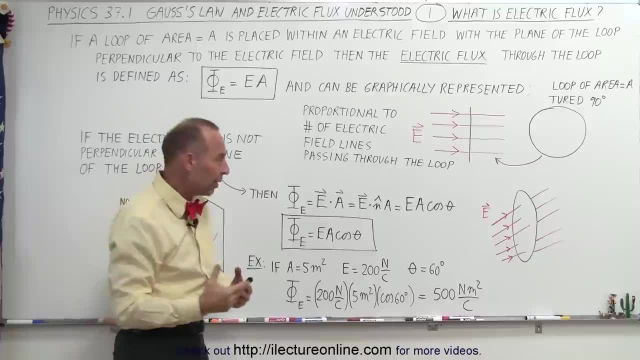 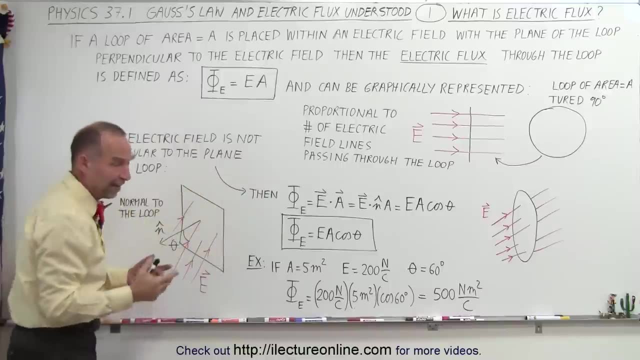 and the area of. now, how can an area have a vector? well, an area can have a vector when you take the normal to the, to the plane. so here we have drawn a loop, and it doesn't have to be a round loop, it can be a square. 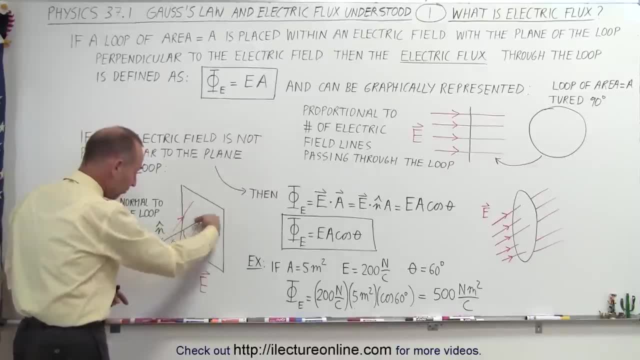 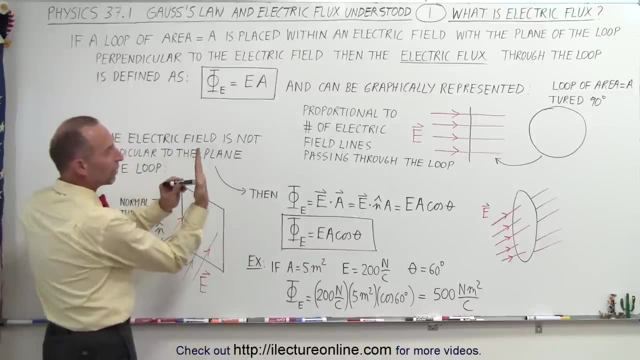 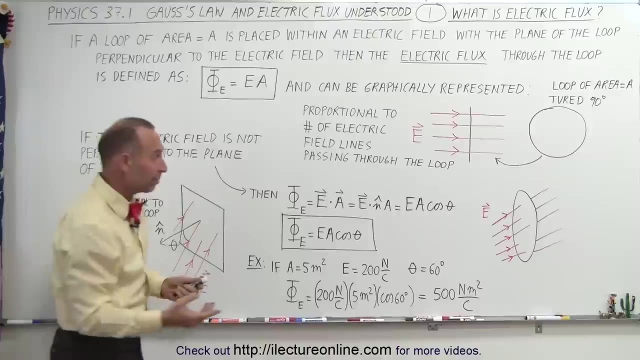 loop. and so here this vector pointing straight out from the, from the loop, from the area, this vector is perpendicular to the plane. so here's the n vector, perpendicular to the plane. and now, if the electric field comes in at a different angle relative to the normal, we can express that by the: 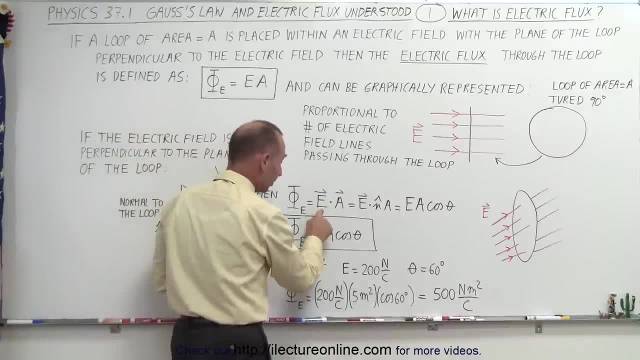 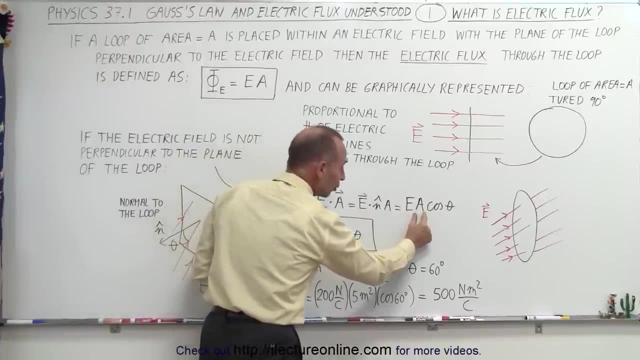 product, it will be the magnitude or not the magnitude, but the electric field times the area, a dot product, which is simply equal to the magnitude of the field times, the area of the loop times, the cosine of the angle between them. so here you can see that if theta represents the 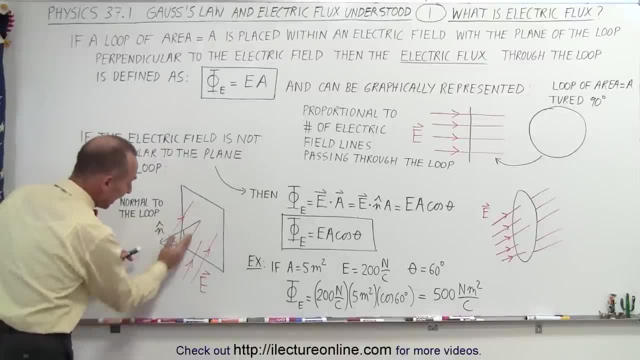 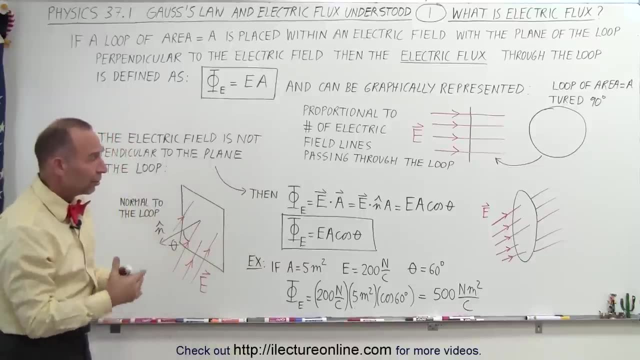 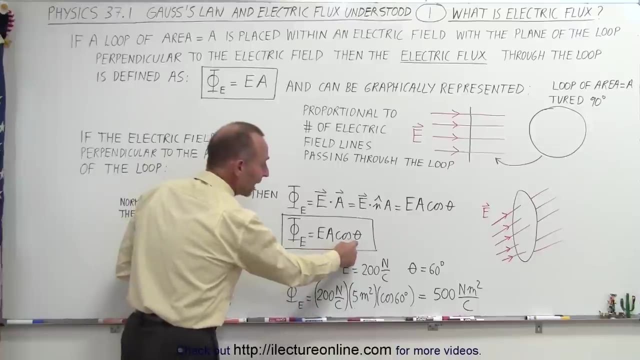 angle between the perpendicular normal vector and the direction of the electric field, then it's simply the size of the or the magnitude of the field times the size of the loop, the area loop times the cosine of the angle between them. So simply we can write it always like this, and of course, if the angle between them is 0 degrees, 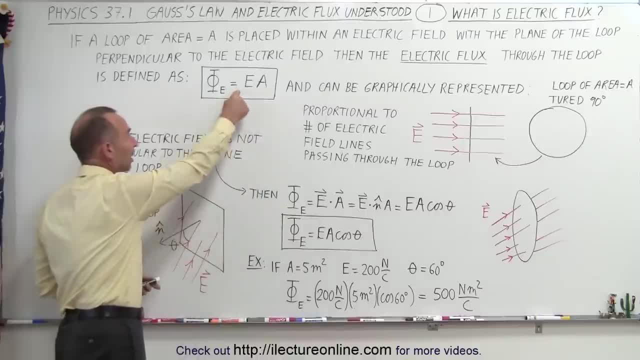 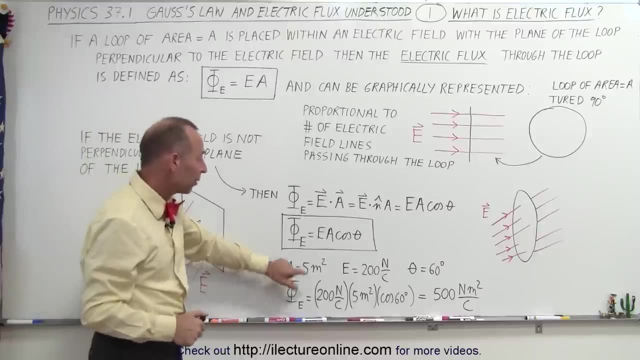 the cosine of 0 is 1, that simply drops out and you come back to the original equation. right here A quick example: let's say that we have an area of a loop that's 5 square meters. The magnitude of the electric field is 200 newtons per coulomb. 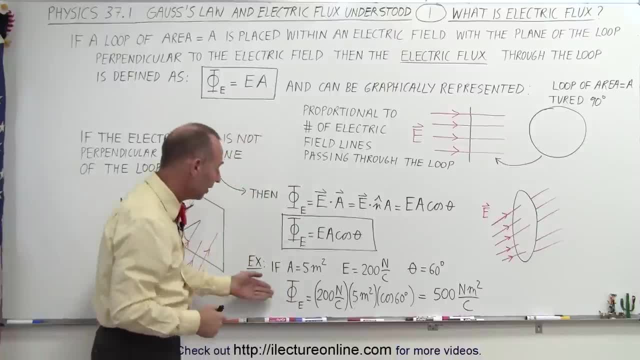 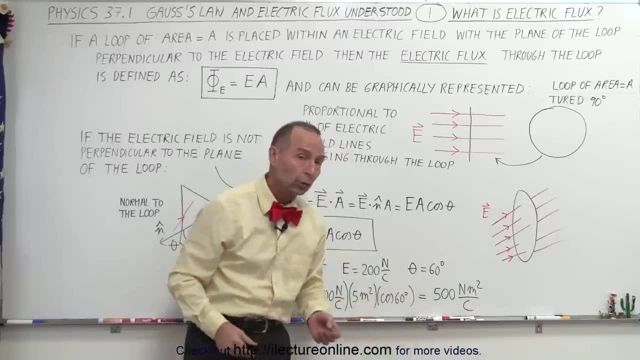 and let's say the angle between the normal and the field is 60 degrees, then the electric flux will simply be the product of all those and that ends up being 500 newton meters squared per coulomb. so you can see that the units for flux or electric flux is newton meters squared per coulomb. 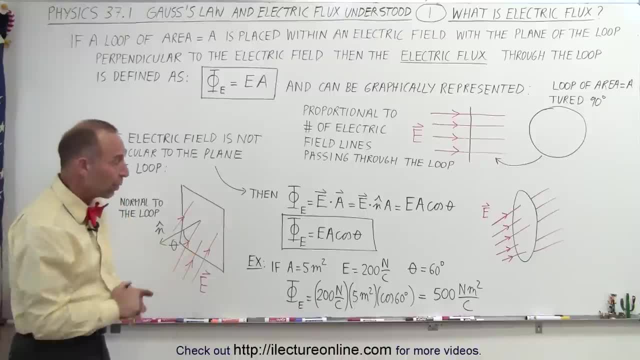 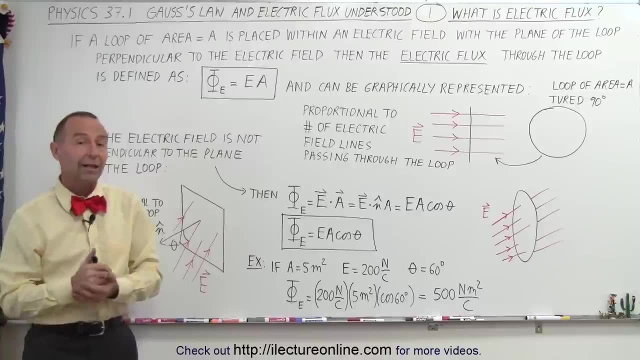 It's newtons per coulomb, the units for electric field and meters squared the units for area, And hopefully that kind of straightens out your understanding about what electric flux is. 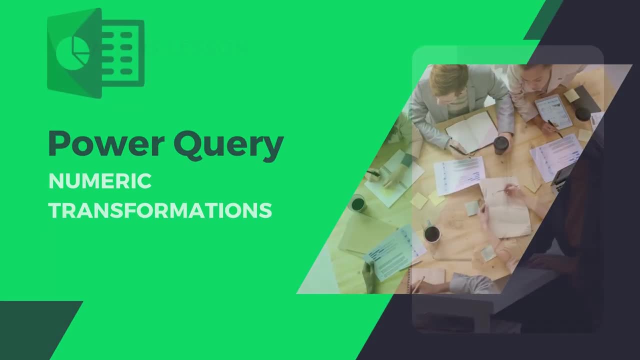 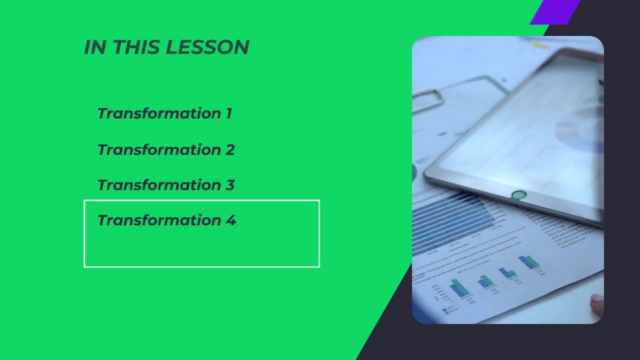 Today we're going to talk about numeric transformations in Power Query. We're going to start off looking at rounding, then we're going to look at arithmetic operations, we're going to look at grouping and aggregation and finally we're going to look at some conditional columns. So let's go. 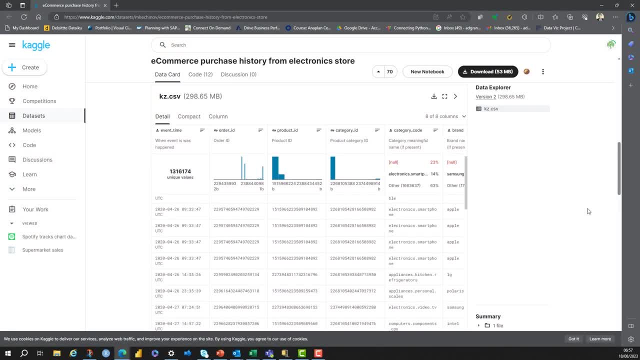 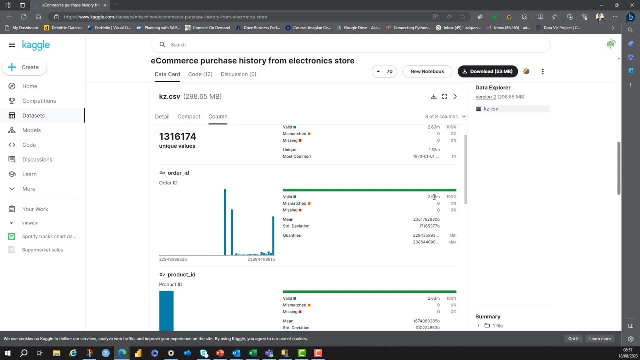 We're going to look at this data set today. This is an e-commerce data set from Kaggle. It has too many rows for Excel, so we've got 2.6 million rows in there, So a perfect data set to try out some Power Query on. 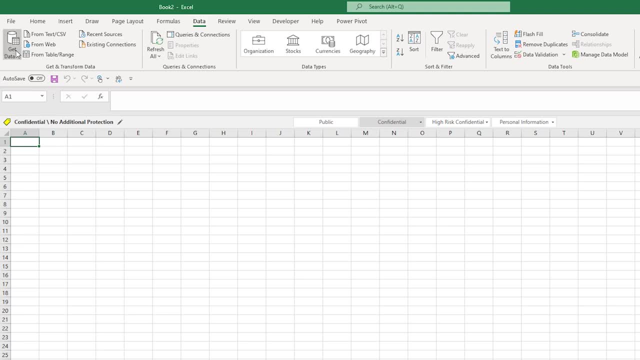 So in Excel, you go to Data, you go to Get Data, you go to From File- and we're working with a CSV today, so From Text CSV. I found my file here which I've downloaded from Kaggle, and then this will load into the preview window. 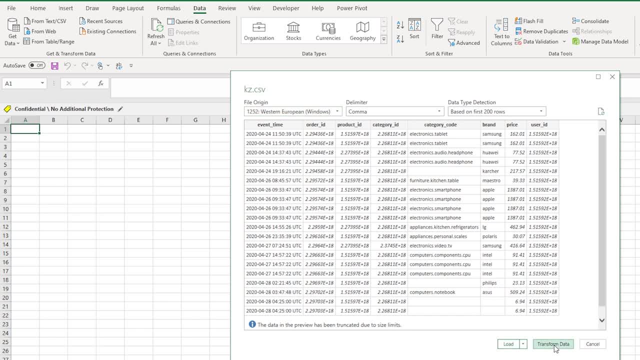 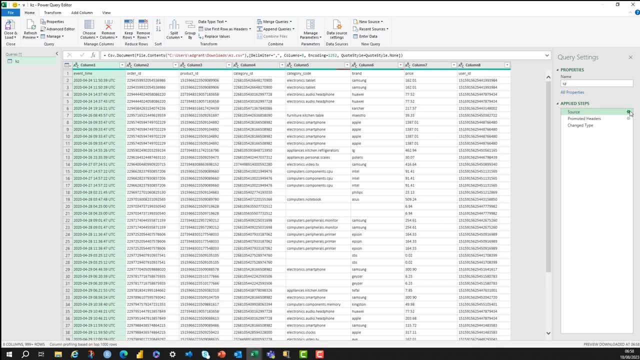 I can not load this to Excel because it's too big, so I'm going to transfer my data to bring it into Power Query. So you might have noticed that there's a couple of steps already done in here. There's the Source step. You can click on the dial here to change any of the steps as they go on. 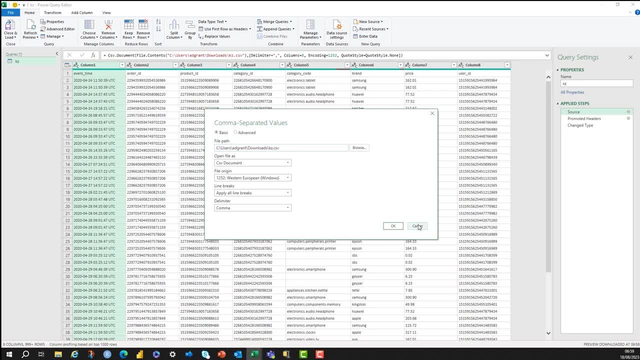 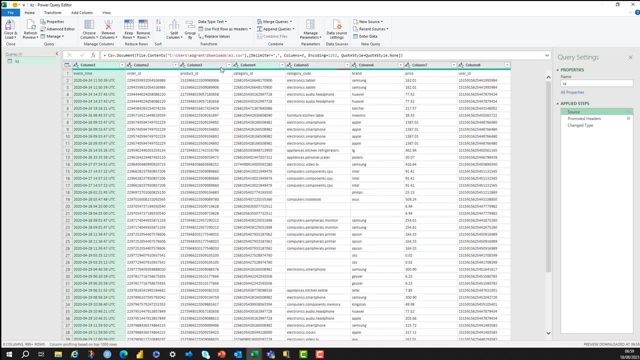 but the source step just defines where the file is coming from, so i can change that at any time. then power query promotes the headers. so you can see they're not promoted in this step here, and then they're promoted in the next step. so that's fine, happy with that. and then power query.